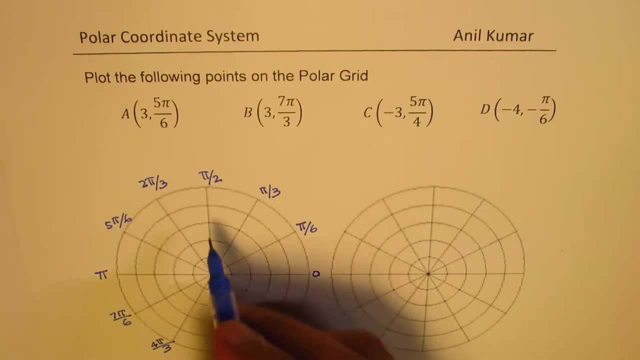 So 7,, 8 and 9 pi by 6, or we get 3 pi by 2, right. So we get 3 pi by 2 here, that is 10 pi by 6.. This is 11 pi by 6, correct. 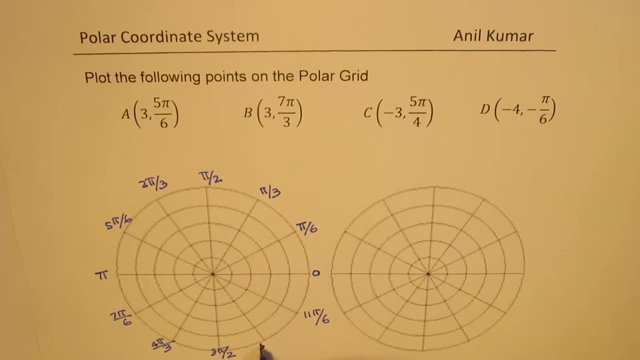 So this is 10 pi by 6. So we get 5 pi by 3, correct. So 10 goes 2, 2 times. So that is what is shown here. Now let's try to. 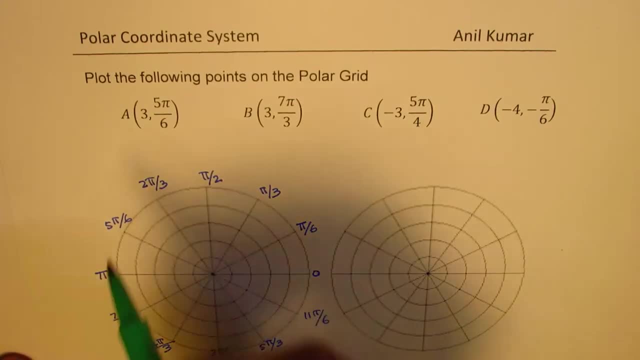 display the information: A is 3,, so radians 3, radians is 5 pi by 6,, now positive. So that means we'll go all the way up to 5 pi by 6.. So what we have here is 5 pi by 6, right there, and R value is 3.. 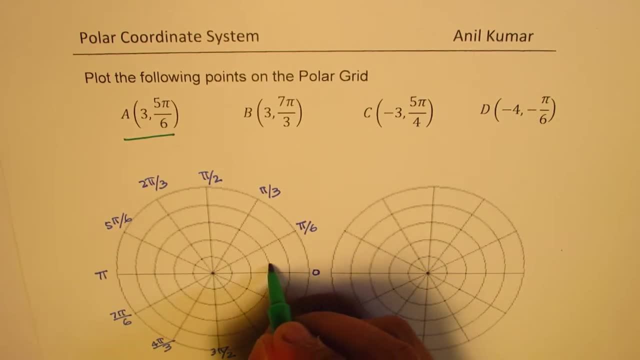 So we go 1,, 2,, 3 units and then go round up to 5 pi by 6. So we reach this place. So that becomes the position right. So we are going to draw it like this. 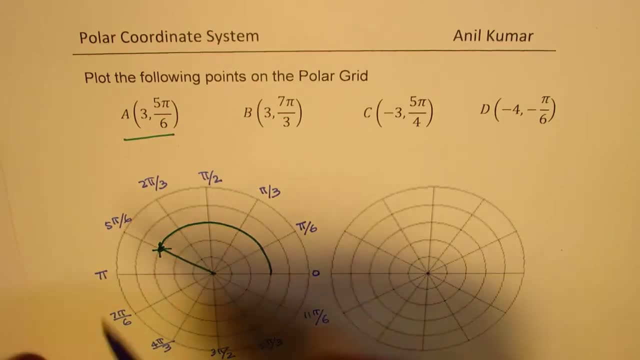 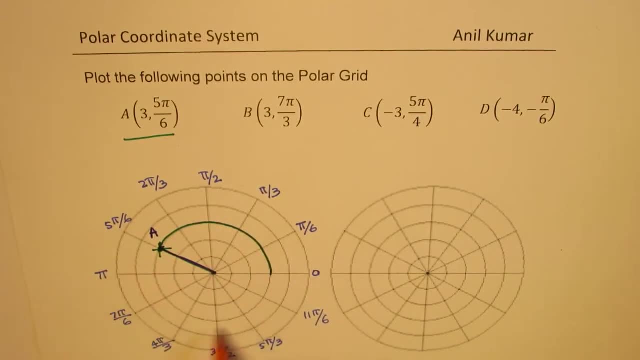 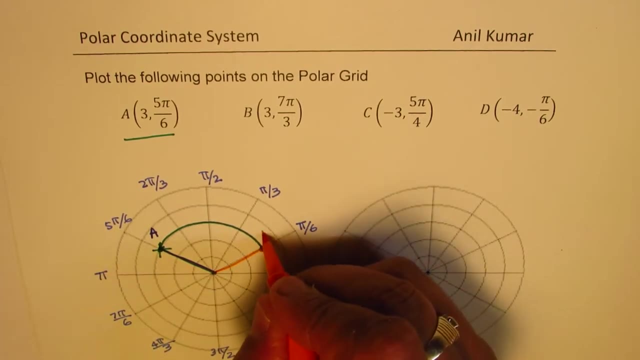 So if you go 3 pi by 3, which is pi 6 pi by 3, and that is 7 pi by 3.. So 7 pi by 3 will be 3 units here and that becomes your point B right. 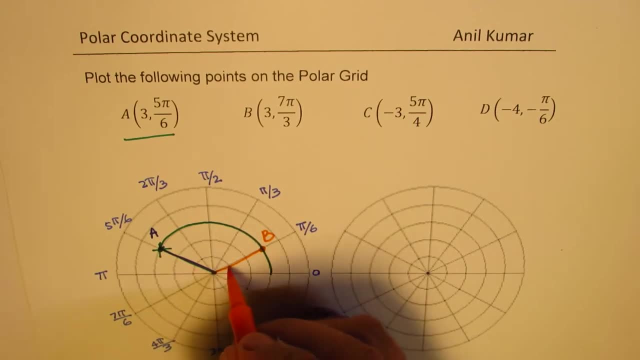 So basically you're going to go round one full circle, 6 pi by 3, I mean going like this, right One full circle and then you'll end up here to 7 pi by 3, is that clear to you? 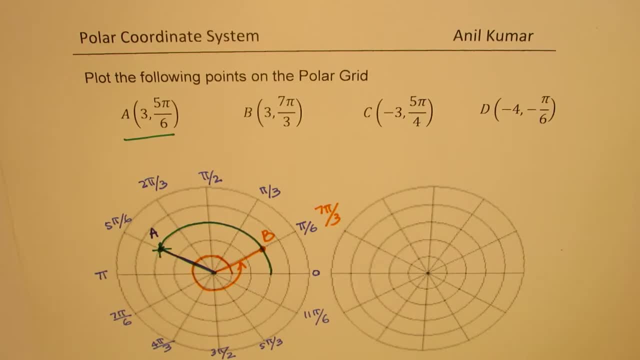 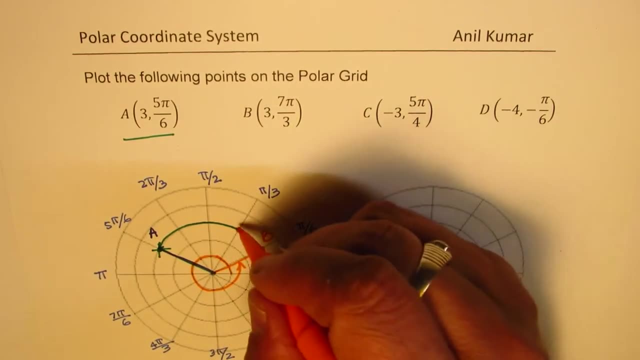 So you'll end up at this position, which matches with sorry 7 pi by 3 will be here, I'm so sorry. 7 pi by 3.. So 6 pi by 3, that will be the position, sorry. 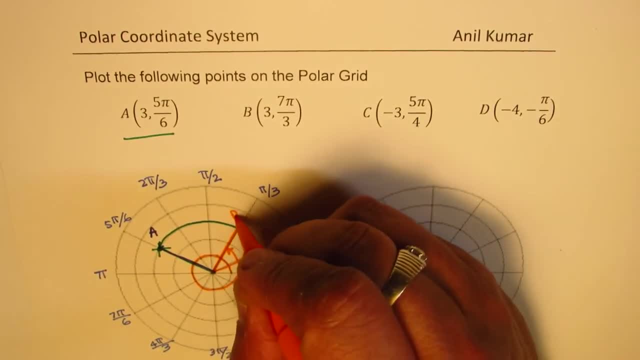 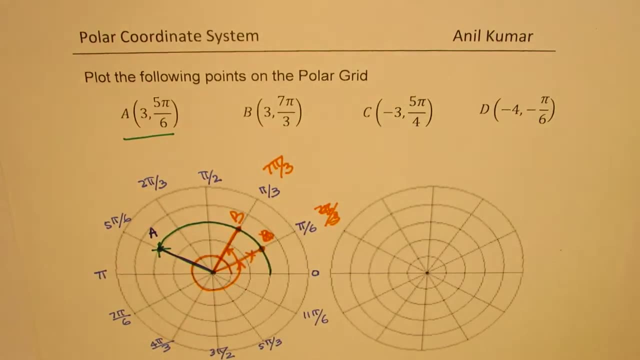 So that becomes 7 pi by 3,, not this. okay, So that is B for us, not this. So that is 7 pi by 3,, okay, Okay. The next one for us is C, which is minus 3.. 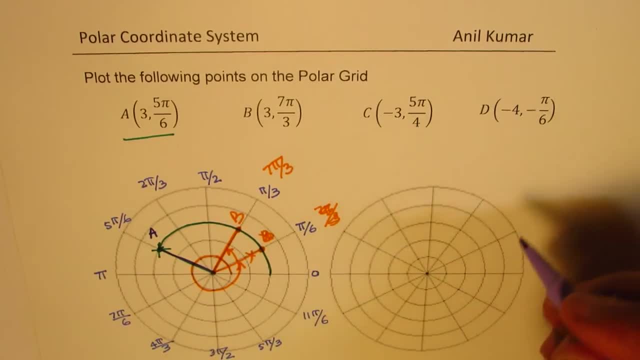 So this is 3, 5 pi by 4, okay. So we're given this in terms of pi by 2, this is 0, right. So when you talk about pi by 4, it is midway, right. 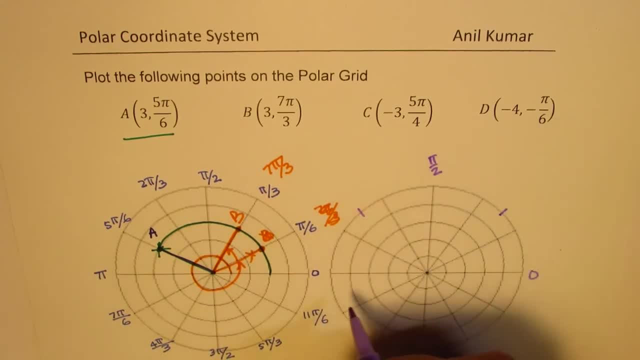 So this is 1 pi by 4, right, This is 2 and this is 3, okay, This is 4, so 5 pi by 4 is here, right, 5 pi by 4, okay. 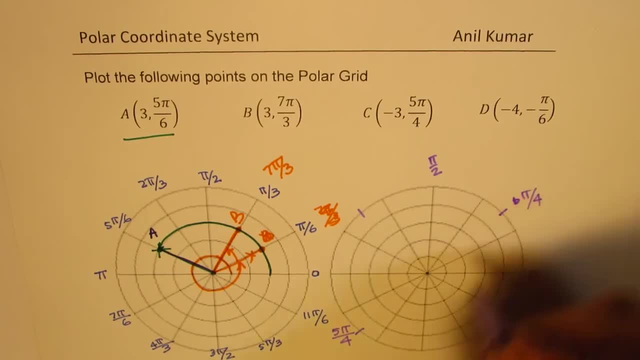 So this is pi by 4.. 2 pi by 4, right 2. pi by 4,, 3 pi by 4, right, 4, pi by 4, 5 pi by 4,. this is 6, and that one right there in the middle. 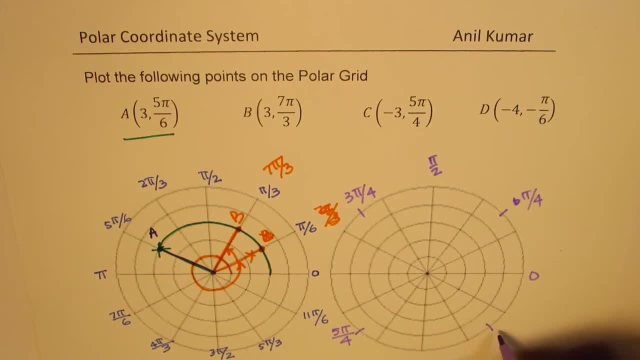 of this diagonally will be your 7 pi by 4, correct, Of course? this is 8 pi by 4.. Now we are going to go to minus 3, 5 pi by 4.. So 3 will be actually in this direction. 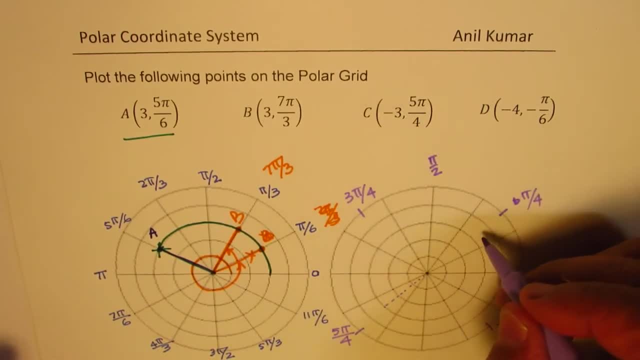 1,, 2,, 3.. But since this is negative, since it is negative, it will point in the opposite direction. So that becomes the point C for us. So if it is negative, then we are taking the point on the other side. It does not point towards the primary angle. okay, So that. 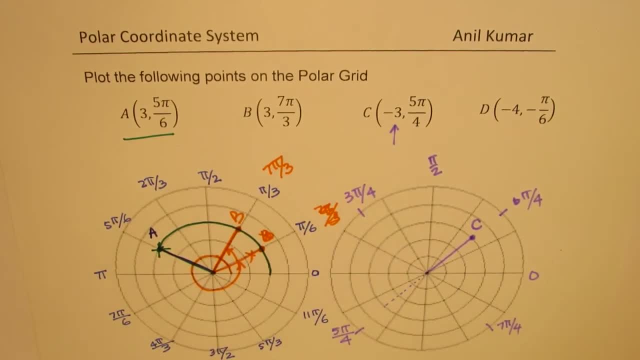 is how we get our negative 3.. Now the last one here is to plot minus 4 minus PI by 6. so let's take care of minus PI by 6 first. so that is minus PI by 6. so you reach here minus 4. we have to go in the opposite direction, right? so?